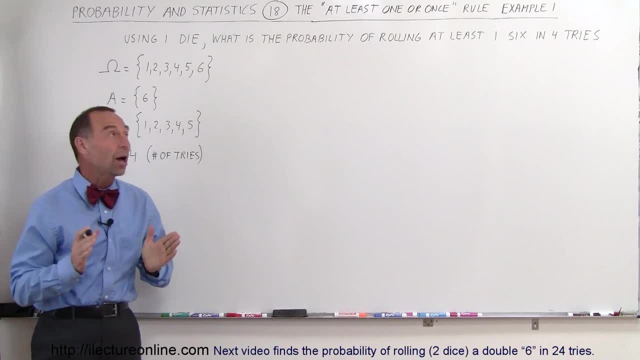 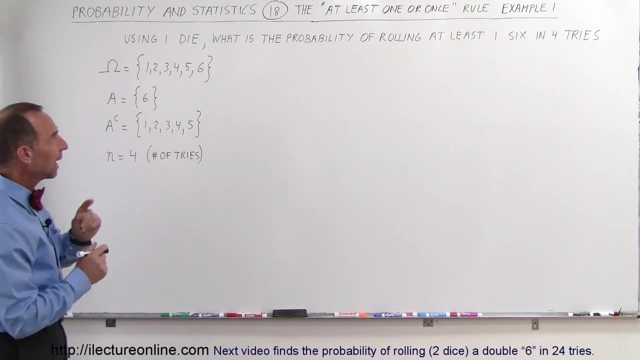 Welcome to. I Like Turnalign, and now we're going to do an example on the what we call the at least one or ones rule. So in this case we have an example where we have single die and we want to know the probability of throwing at least one six. 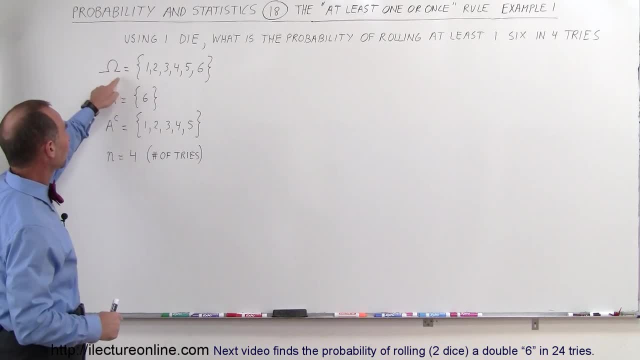 in four attempts. Alright, so the sample space is, of course, all the numbers on the die. the event that we're trying to achieve is the number six. the complement of that is, of course, all the other numbers, and the number tries is 4, so &. 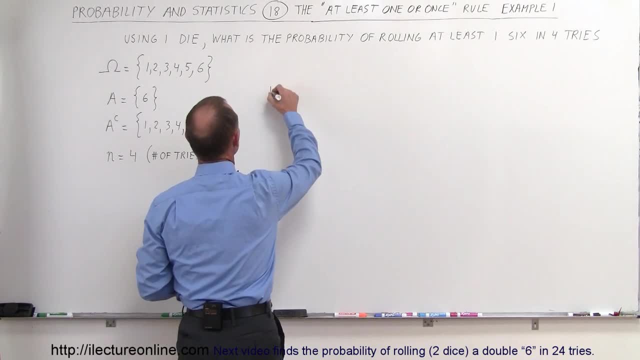 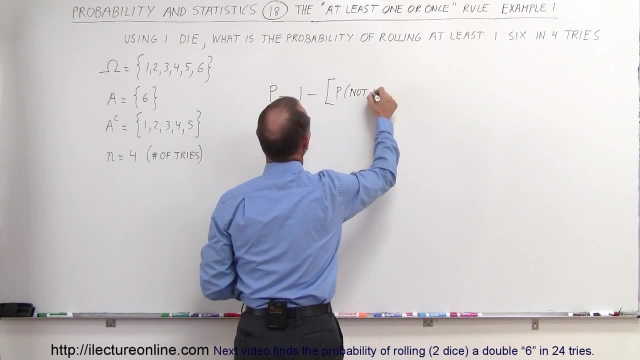 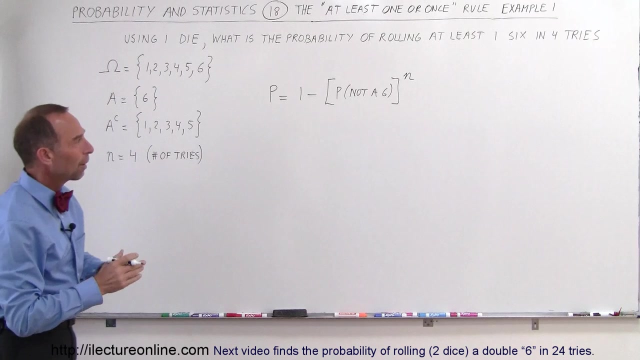 equals 4 and the equation we use for that is the probability is equal to 1, minus the probability of not getting a 6 raised to the n-th power, for that number tries And, of course, the probability if not a six. that would be the complement. 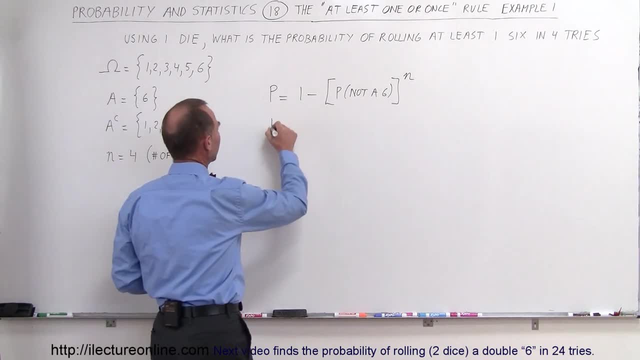 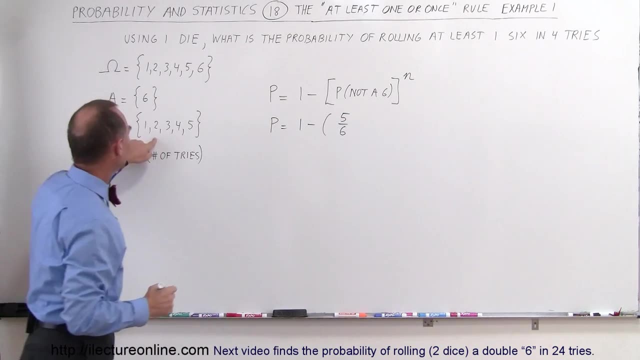 of a Alright. so that means that the probability is equal to 1 minus. that would be 5 over 6 because the complement the other numbers would be 5 out of a total of 6 in the sample space and then raised to the 4th power. 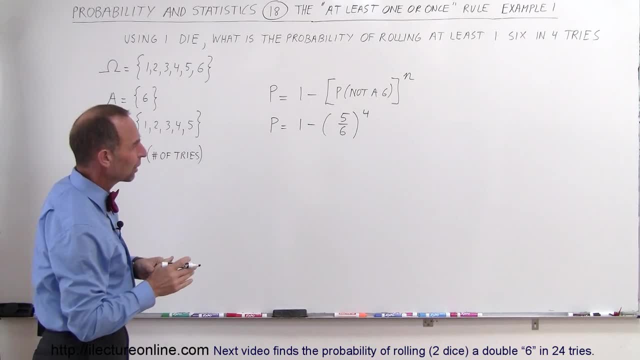 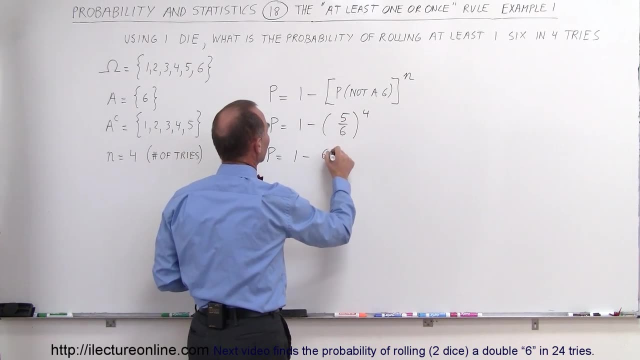 Now here. you might want a calculator. you may want to try to do it without a calculator. I don't know if we can. So probability is equal to 1 minus 5 to the 4th power, that would be 625,. 6 to the 4th power, that's 216, that's 12,, that's 1296, I believe it is. 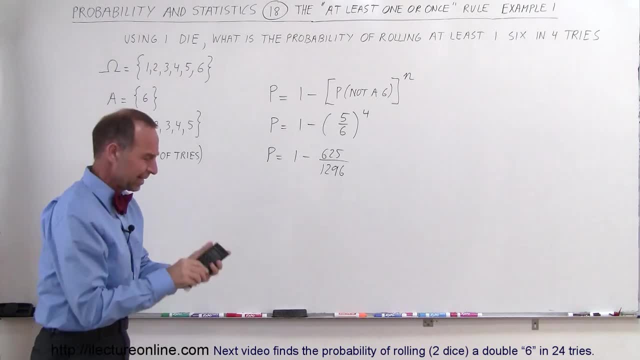 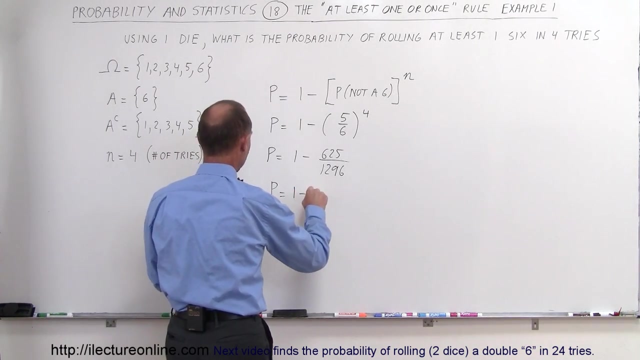 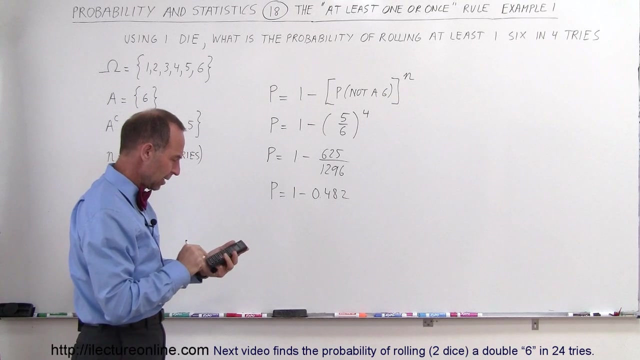 Okay, I'll probably verify that with my calculator. Alright, and so we have 6 squared squared. yep, that's correct. take the inverse of that times 625.. And so that would be equal to the. So probability is equal to 1 minus 0.482, of course, when we subtract that from 1, we get the probability is equal to 0.518.. 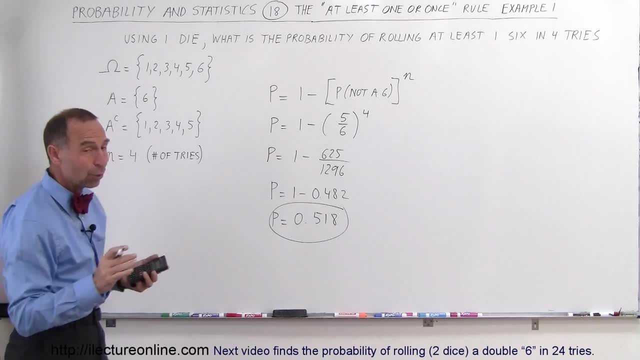 So that's interesting. you may not have thought so, but if you throw a die, 4 times the probability of getting any one number- not just 6, but any one number- is better than 50-50.. You're better than 5..